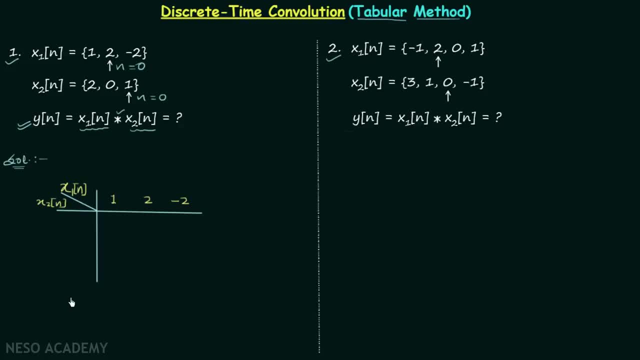 second discrete time signal: X2n: vertically: 2: 0, 1, 2, 0, 1.. Now focus on the method. We will obtain our first row by multiplying the first element of X2n by all the elements of X1n. So 2 multiplied to 1 will give us 2, 2 multiplied to 2. 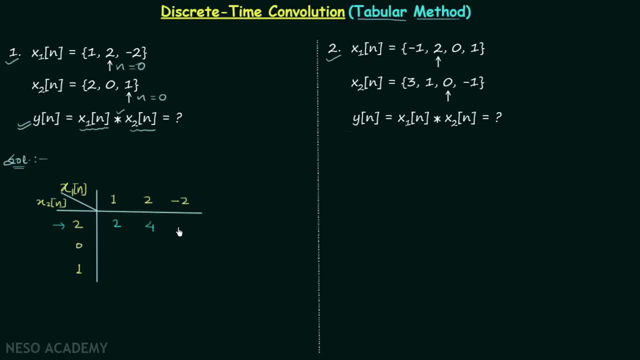 will give us 4,. 2 multiplied to minus 2 will give us minus 4.. Pretty easy, Now let's obtain our second row, and we will multiply now the second element of X2n by all the elements of X1n. Now let's write down the values of signal X2n. 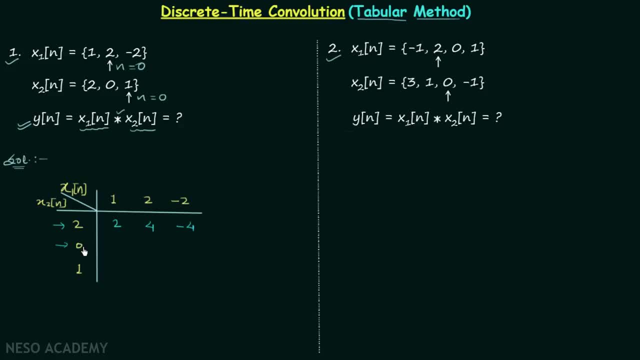 לנו 2 minus 2, and now we will obtain the elements of X2N by all the elements of X1n. When you multiply 0 to 1,, 2, 2 to minus 2, you will get 0.. Following the same process to get the third row. 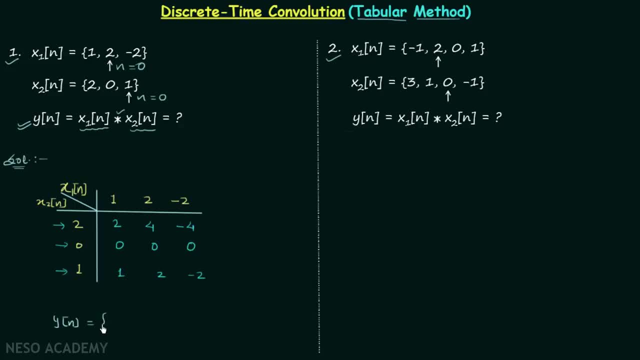 of signal yn. To get the elements of signal yn, we will perform the addition diagonally, So you can see that 2 is alone here. There is no other element diagonally with 2.. Therefore we will write 2 as it is. After this, we will add 0 and 4.. 0 plus 4 is equal to 4.. Then 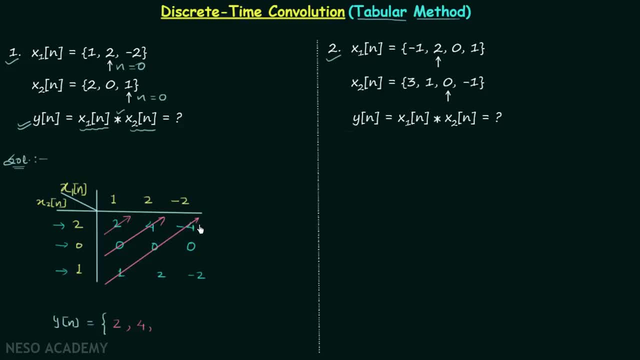 we have 1 plus 0 plus minus 4.. 1 plus 0 plus minus 4 is equal to minus 3.. After this we have 2 plus 0, which is 2, and then finally this minus 2 is alone. so we will write minus. 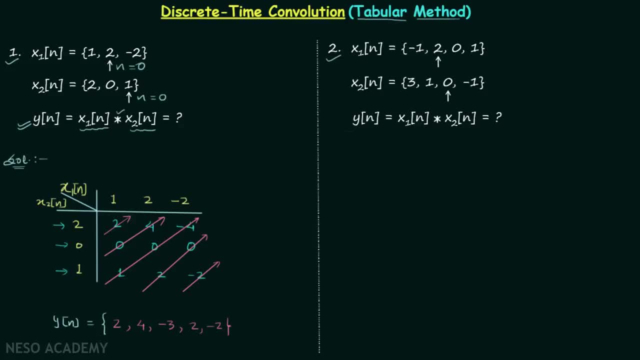 2.. So these are the elements of our signal yn, and now we will focus on obtaining the element which is present at n equal to zero. Because? Because without defining the element present at n equal to zero, we don't have the complete information about signal yn. 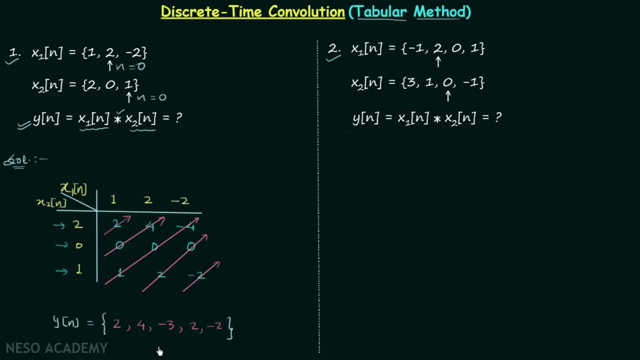 So let's understand how to get the element present at n equal to zero. For that we will focus on the elements of x1n and x2n present at n equal to zero. You can see that x1n is having 2 as the element present at n equal to zero, and x2n is having 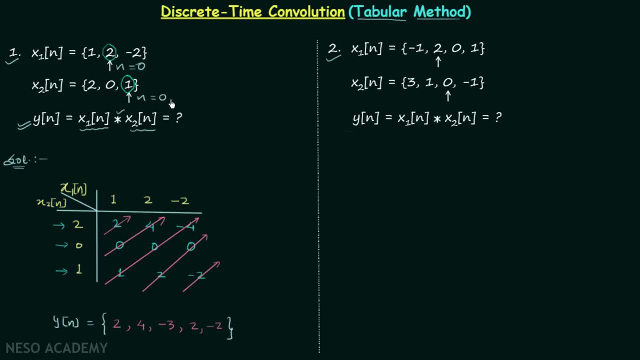 the 1 as the element present at n, equal to zero. So what we will do, we will draw a vertical line passing through 2 and we will draw a horizontal line passing through 1, and you can see that this is the point of intersection. 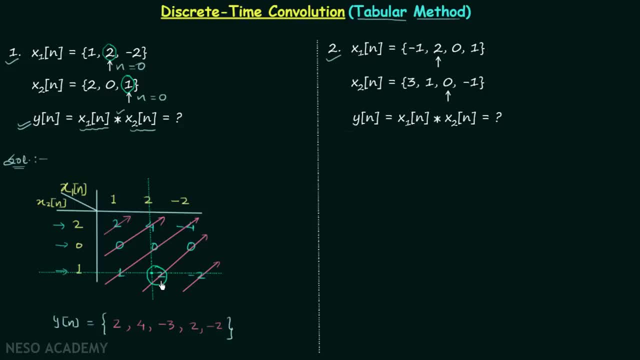 and at this point we are having 2. 2 as the value in the table and this 2, when added with zero, is giving us 2.. So whatever value you are getting after the addition of this element, you will put your arrow below that value. 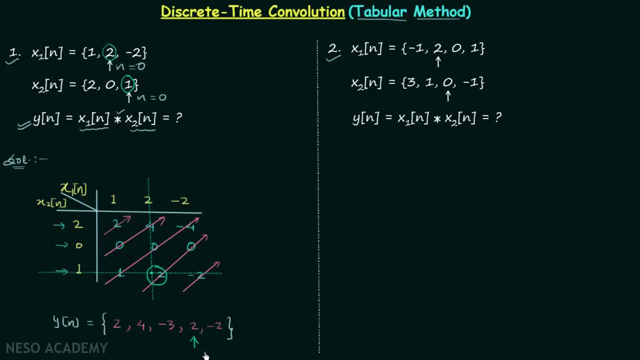 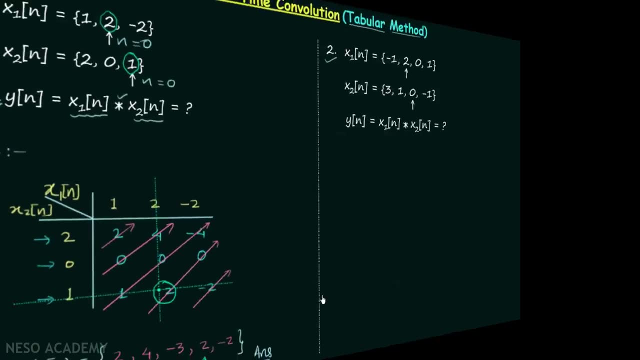 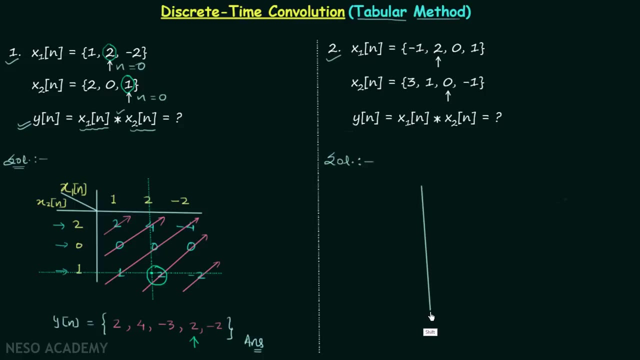 So 2 is the value of yn when n is equal to zero. So this is our answer. Now let's move on to the second example. So let's move on to the second example. We will first draw the table and we will write down the values of signal x1n horizontally. 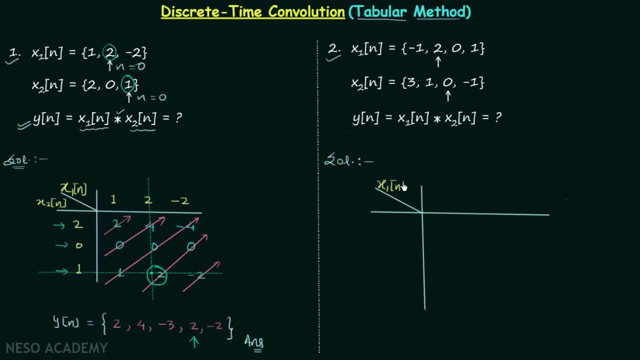 We will write down the values of discrete time signal x1n horizontally Minus 1,, 2, 0, 1.. Minus 1,, 2, 0 and 1.. After this, We will write down the values of signal x2n vertically: 3, 1, 0, minus 1, 3, 1, 0 and minus. 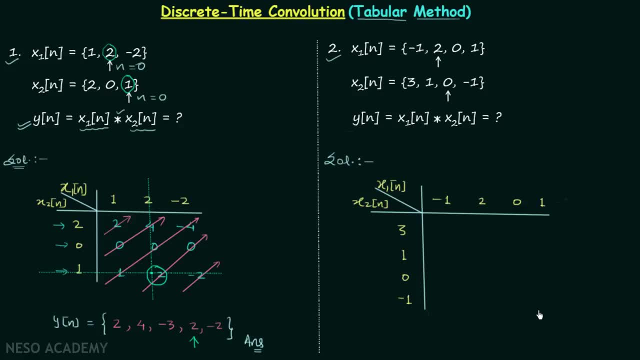 1.. Now let's obtain the rows of the table. To get the first row, we will multiply 3 to minus 1,, 3 to 2, 3 to 0 and 3 to 1.. This will give us minus 3,, 6,, 0 and 3.. 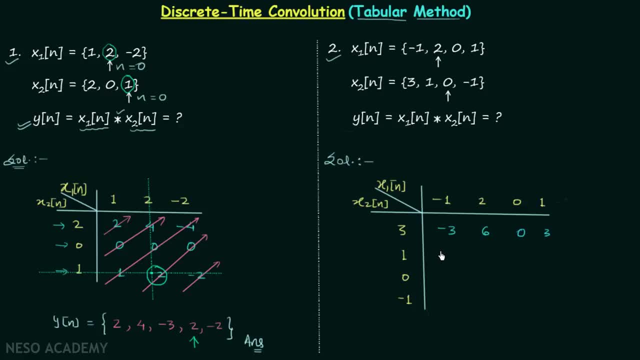 After this, We will obtain the second row, And for that we will multiply 1 to all the elements of x1n. This will give us minus 1, 2, 0, 1.. And the third row will be 0, 0, 0, 0 and the final row will be 1, minus 2, 0, minus 1.. 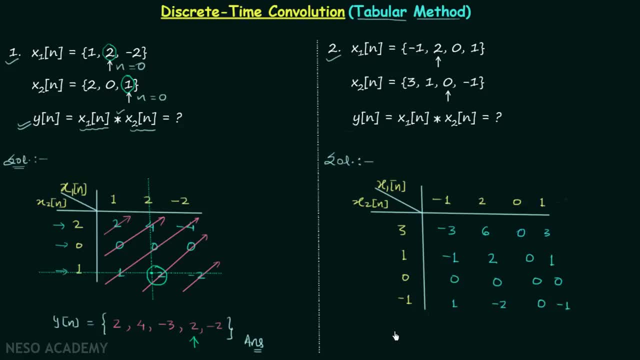 Let's write down The samples of signal yn. Then write down the values of x1n. The third row will be 0, 0, 0, 0 and the final row will be 1, minus 2, 0, minus 1.. 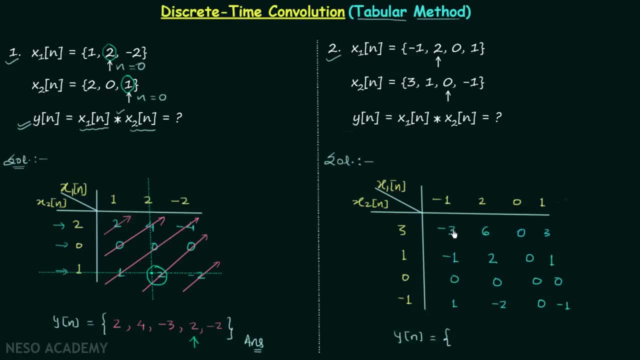 n. We will have minus three, then we have minus one plus six, that is five. After this we have zero plus two plus zero. this means two. then we have one plus zero plus zero plus three. this means four. then we have minus two plus zero plus one. this will give. 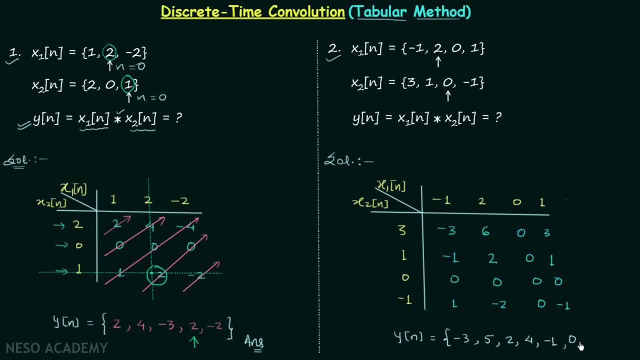 us minus one. then we have zero plus zero, giving us zero, and finally we have minus one. Now we will get the value of the signal Yn when n is equal to zero, And for that we will locate the value of signal X1n when n is equal to zero. that is two, this two here. 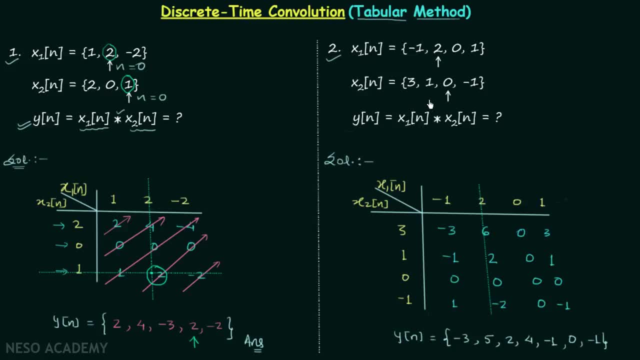 After this, we will locate the value of signal X2n when n is equal to zero and the value is zero. So you can see that we are getting the intersection point as this one and this is the element at the intersection point. So one plus zero plus zero plus three is giving us four and we are getting this result after. 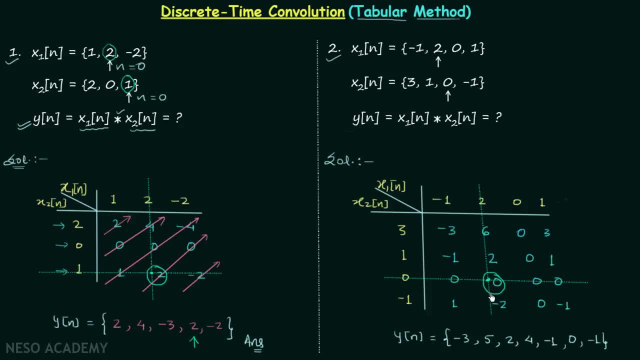 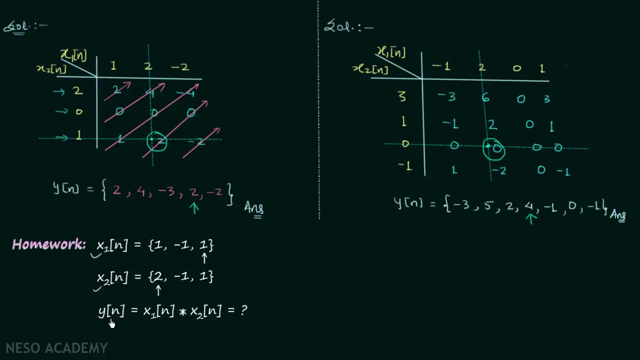 adding the element at the intersection point. Therefore, four is the value of signal Yn when n is equal to zero. So this is the final answer. and now, after obtaining this answer, we will move on to the homework problem. In the homework problem, you can see that two signals are given and you need to find Yn. 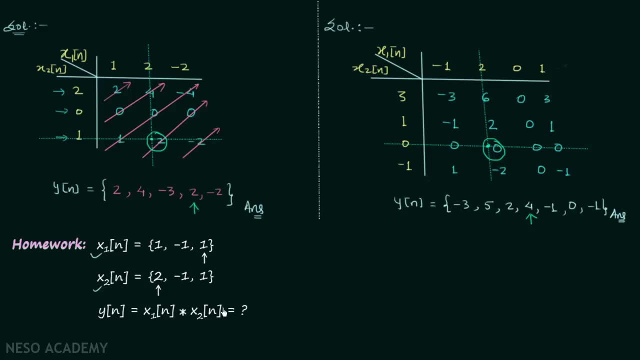 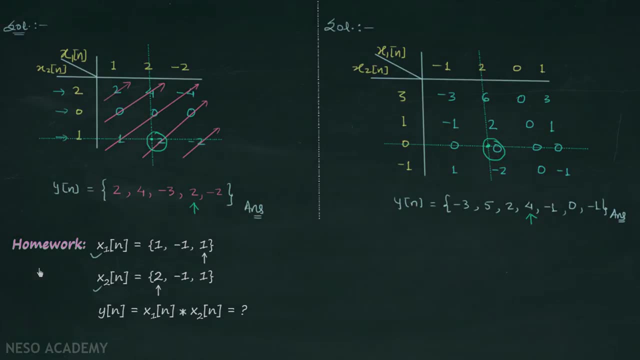 which is equal to convolution of X1n and X2n. So solve the homework problem And once you have your answer, Post it in comment section.